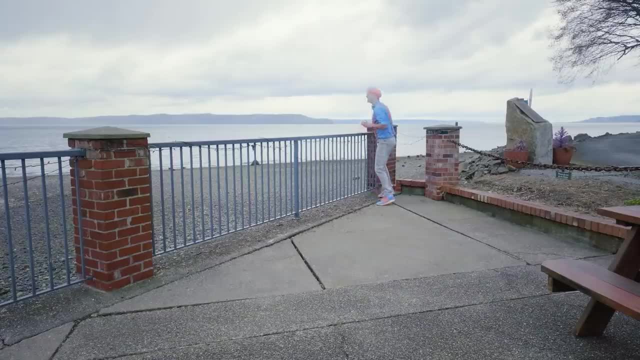 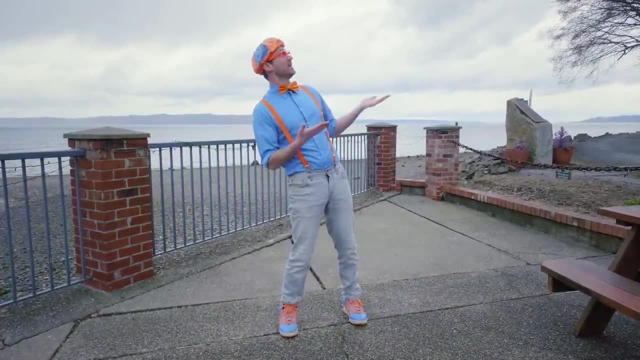 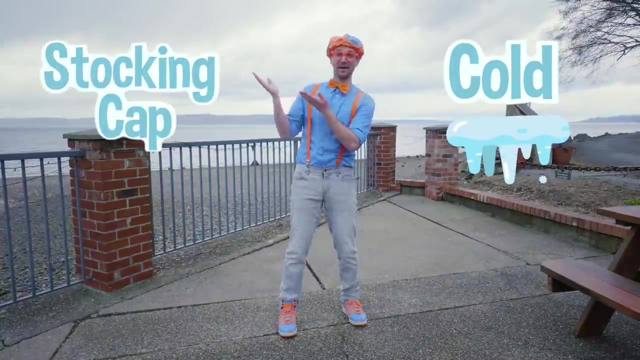 Wow, Weather can sure be very unpredictable, Yeah, Hey, if it's sunny you might need a tank top, If it's cold you might want a stocking cap, But if it's about to rain, you definitely want some rain gear on. 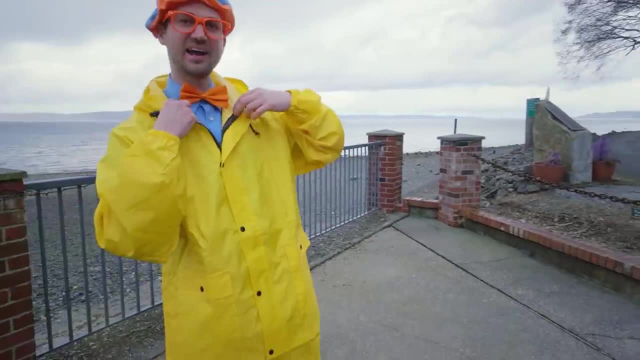 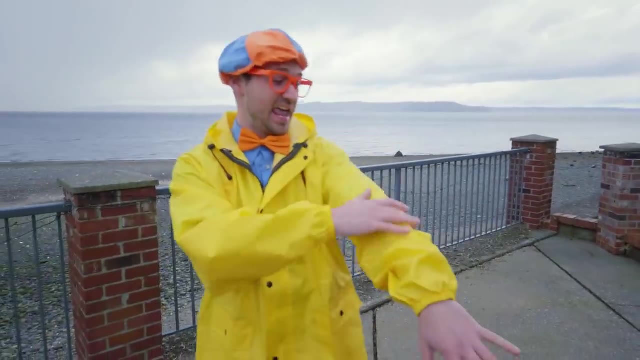 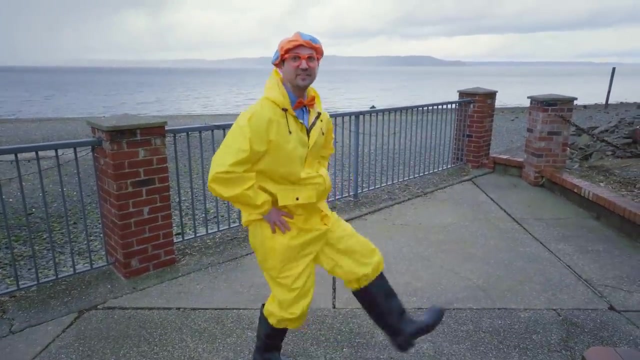 Woo-hoo-hoo-hoo, Check it out. Yeah, I got my rain jacket on. Whoa, it's fully waterproof. So even if it pours down tons of rain, yeah, I will stay really dry. And I got my matching bottoms on. Yeah, what color's my outfit? 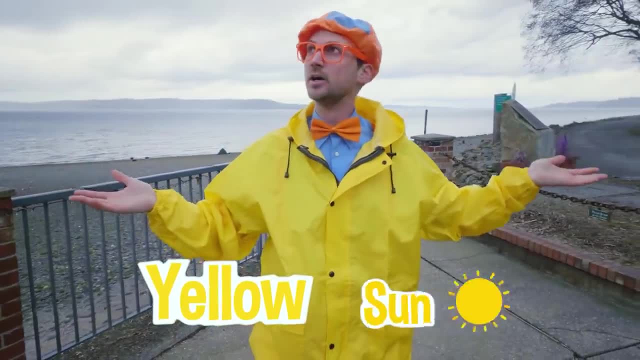 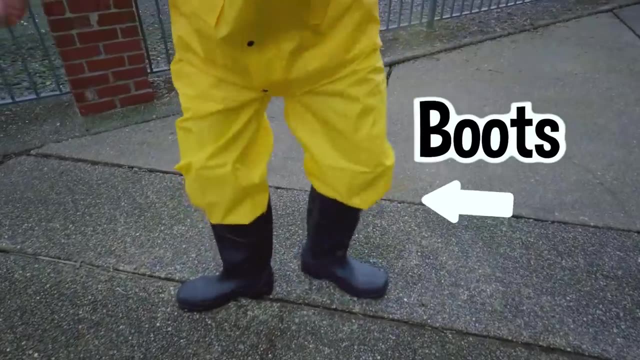 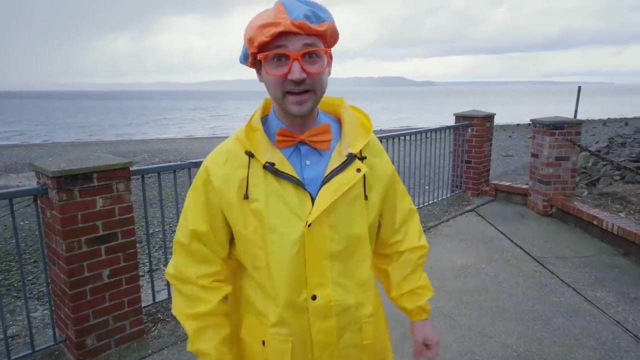 Yeah, it's the color yellow, just like the sun. Where's the sun, I don't know. But hey, check out my boots. Yeah, I have black rubber boots on. And the last thing that I'm missing. yeah, let's go find an umbrella. 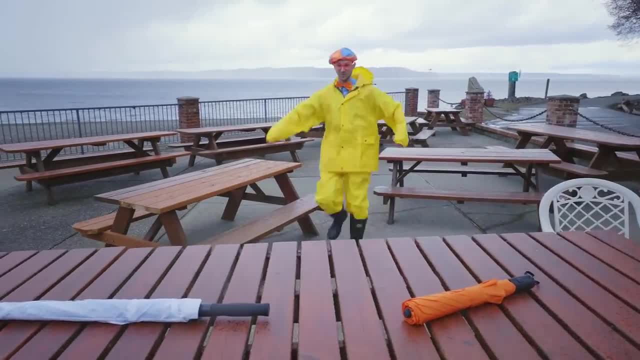 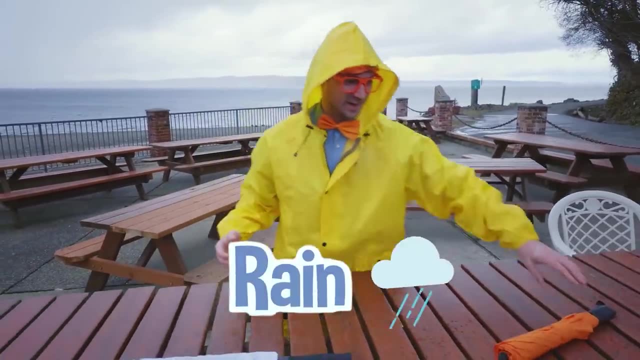 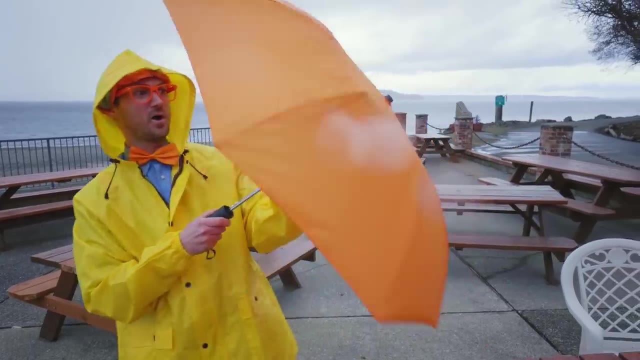 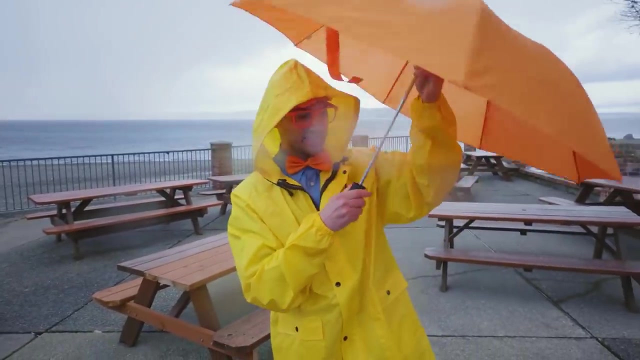 Whoa, Okay, let me put my hood on. Wow, it's really starting to rain. All right, check it out. An orange umbrella, Let's open it up. Whoa, Now there's no rain hitting me at all. Wow, Okay, let's put this one away. 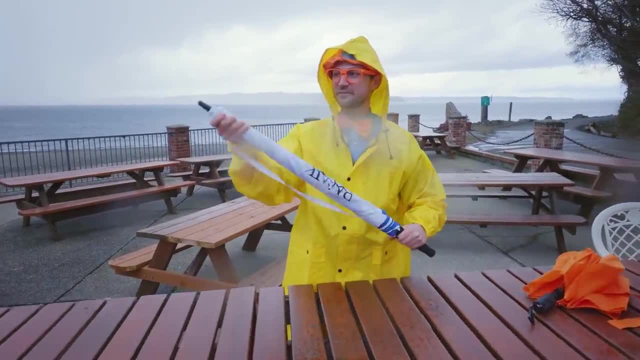 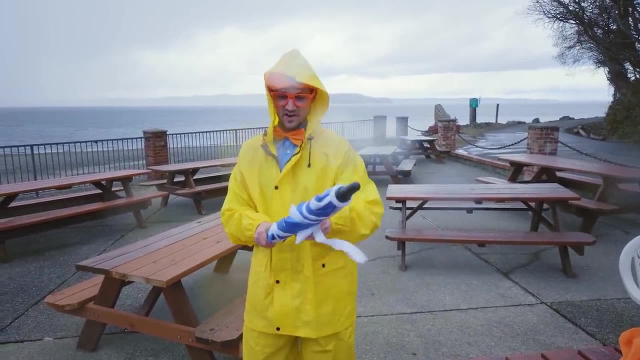 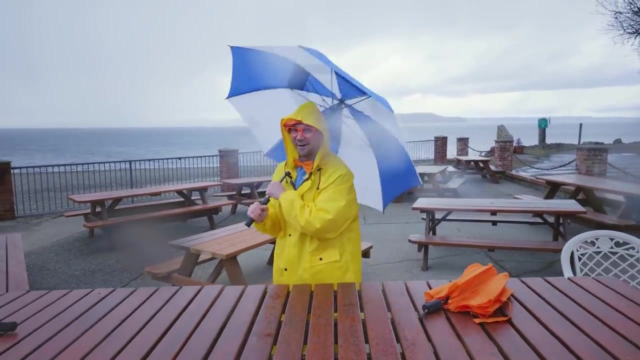 Okay, what's this next one? This umbrella was really small And this one, whoa, is so big. Whoa-ho-ho-ho-ho-ho, Whoa, check it out. Whoa-ho-ho-ho, Woo-hoo. 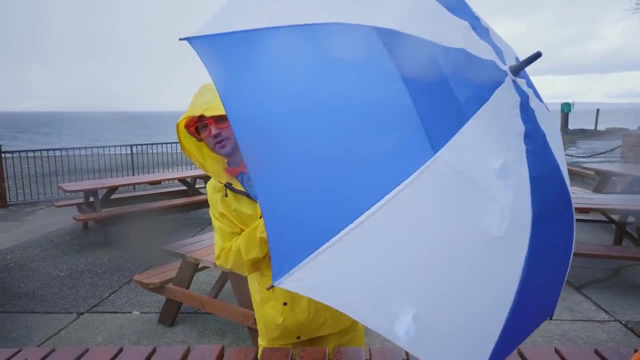 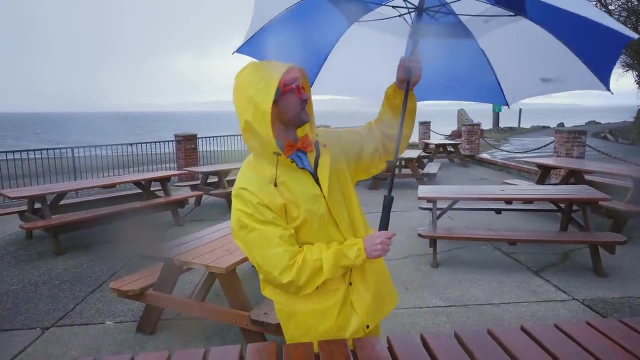 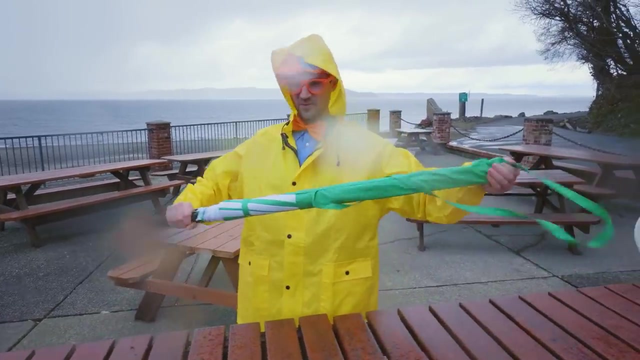 What color is this umbrella? Yeah, blue and white. Woo-hoo, Wee. Okay, let me put this down before I fly away. Oh, okay, And for this umbrella? whoa, Check it out. Yeah, another big umbrella. 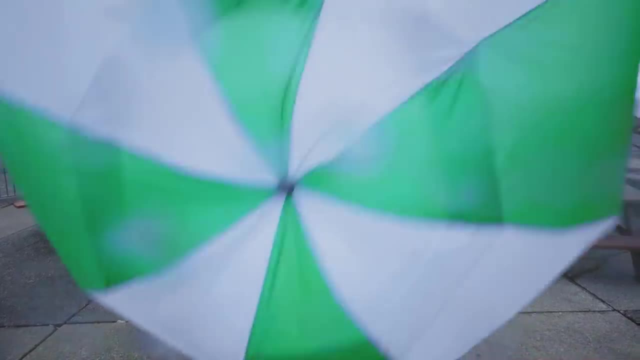 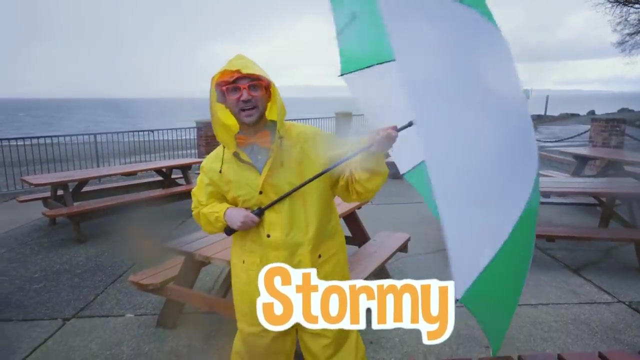 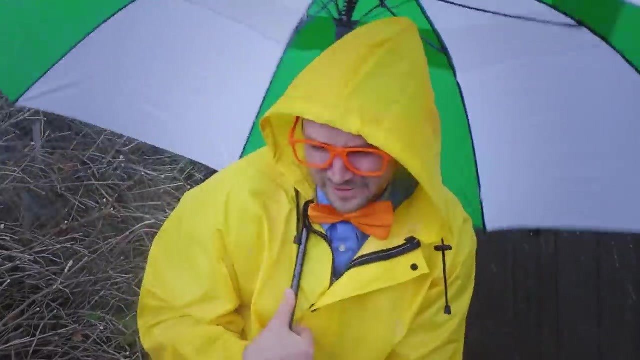 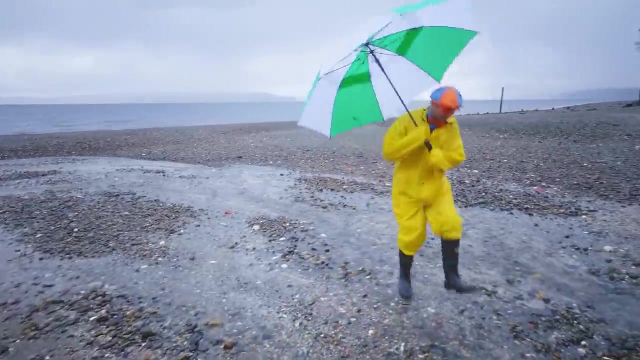 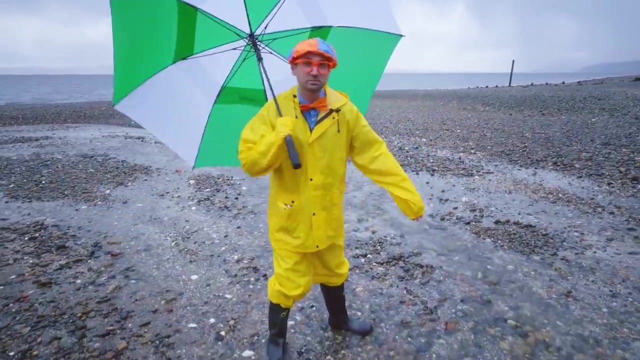 And the colors of this umbrella are: Whoa, It is so stormy out. Yeah, It is white and green. Woo-hoo, Let's go. Wow, I love the rain. The cool thing about rain gear is you can even splash in the puddles and streams that were created by the rain and you won't even get wet. 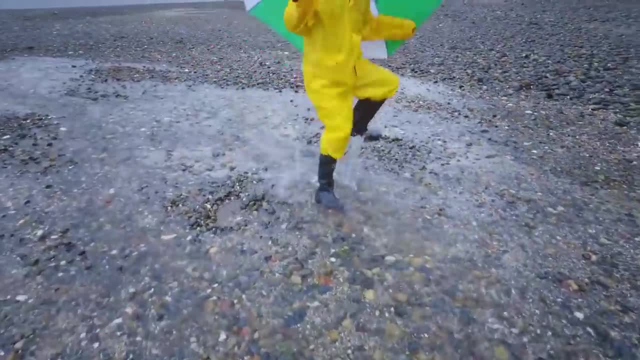 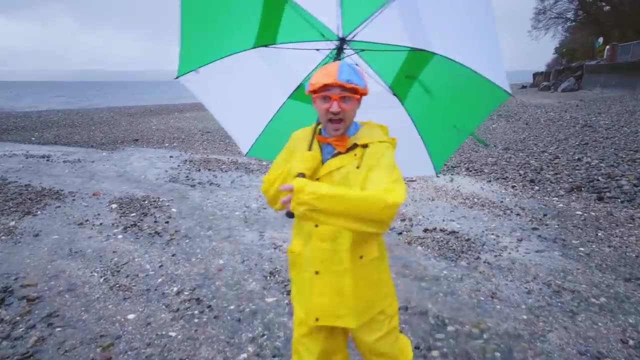 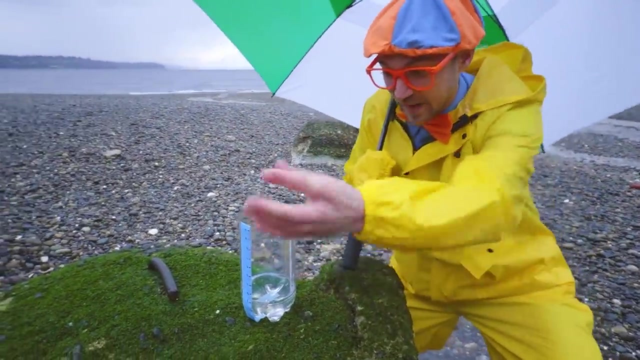 Ha-ha-ha, Woo-hoo, Woo-hoo-hoo-hoo, Yeah, Yay-hee-hee-hee. Hey, check it out. Look back here. Wow, Do you see this? Yeah, this is my rain collector. I set this out earlier, before it started to rain. 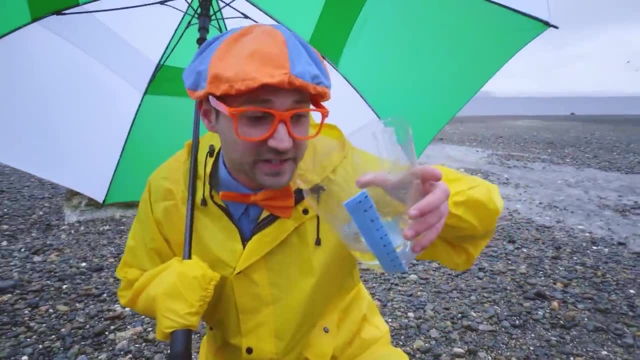 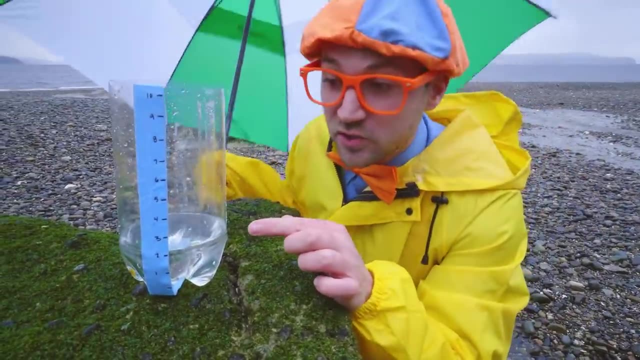 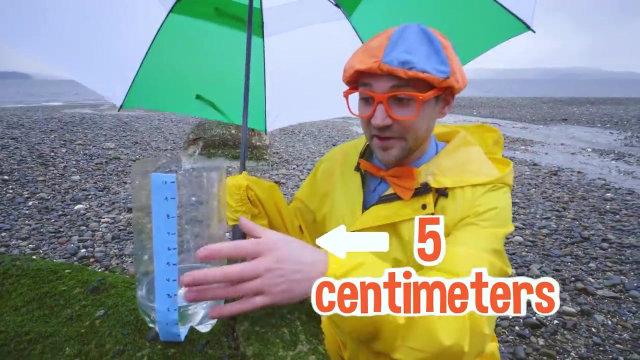 And then all this rain collected from the top. Do you see how much it says Wow, Yeah, it says about two inches. Yeah, that's just over five centimeters of rain. Wow, Wow, That's a lot of rain. 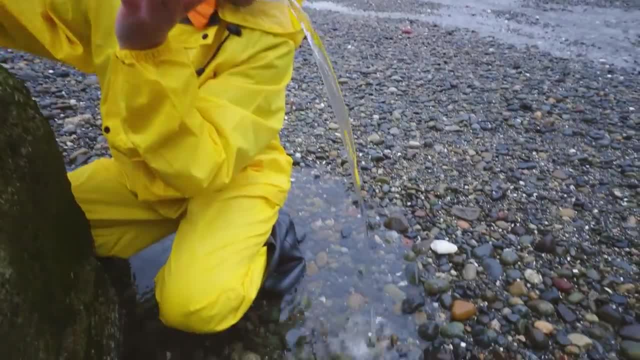 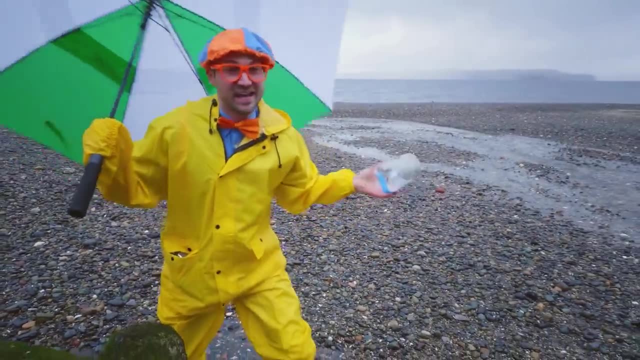 Okay, I'm going to pour it back Yep Onto our planet Earth, Because when the rain falls on our planet, it's really good for it. It helps keep all the plants nice and moist and our oceans nice and full. 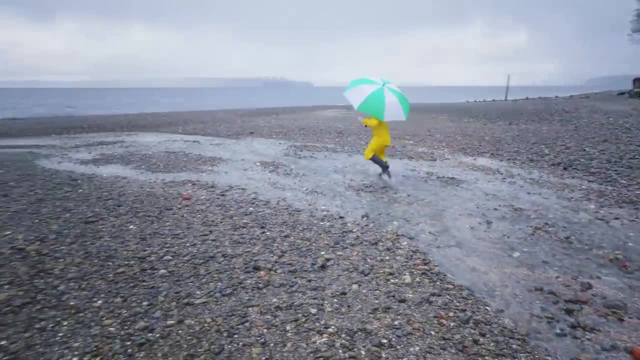 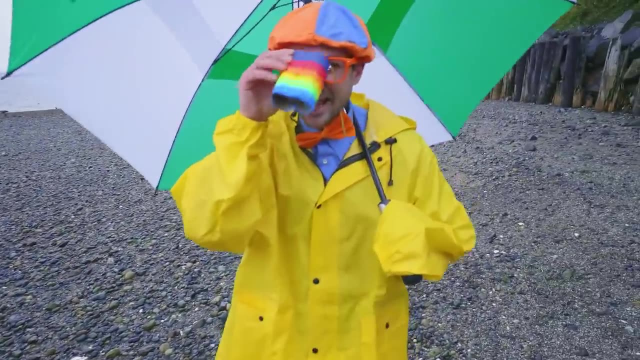 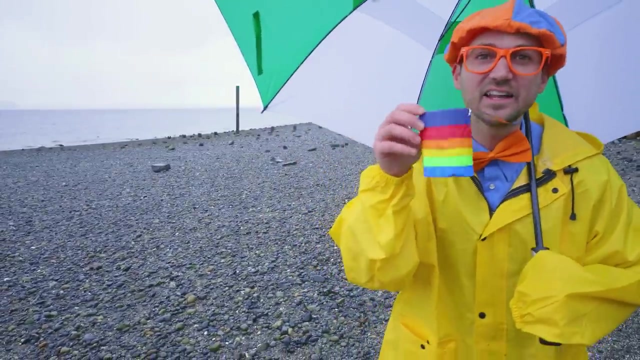 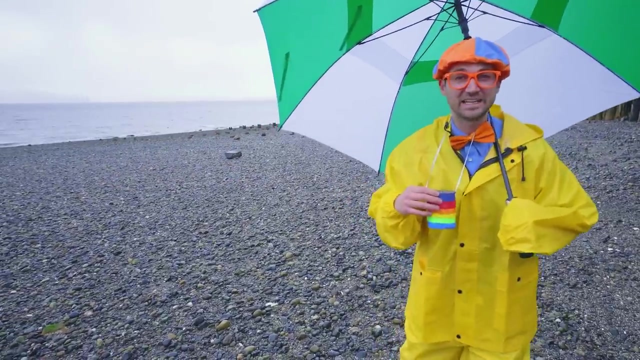 Ha-ha, Woo-hoo. Hey, Check it out. Yeah, These are my rainbow oculars. Yeah, Isn't that cool? Yeah, they're the colors of the rainbow. Have you ever seen a rainbow before? Yeah, they love to come out after it rained. 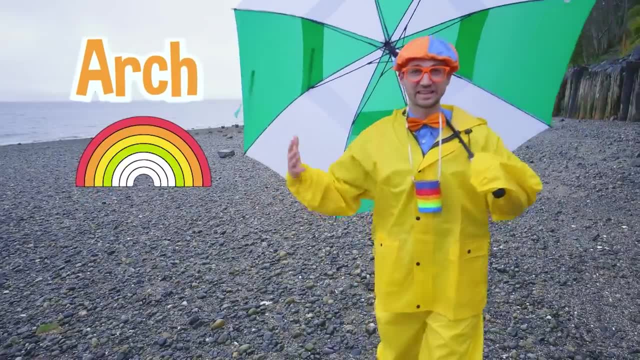 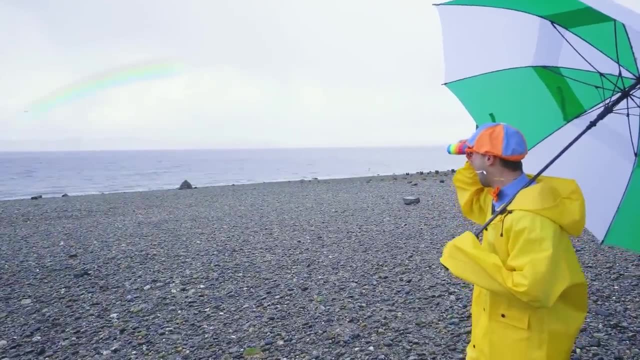 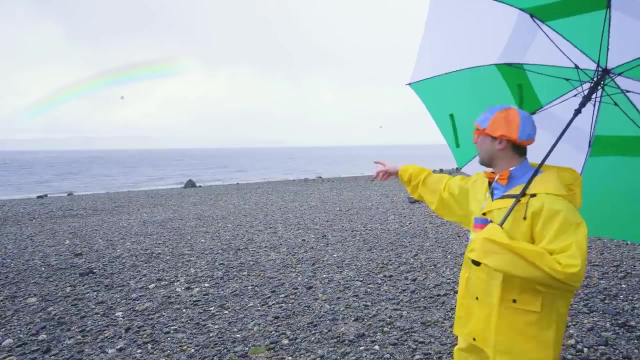 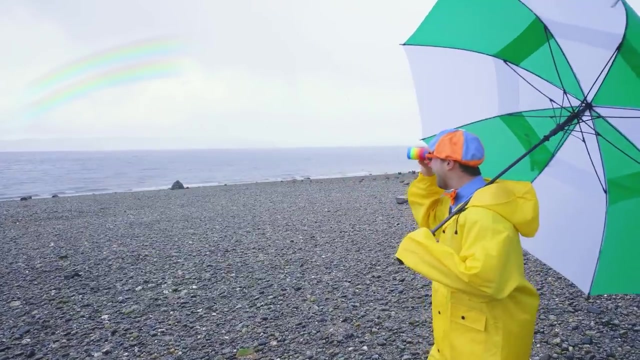 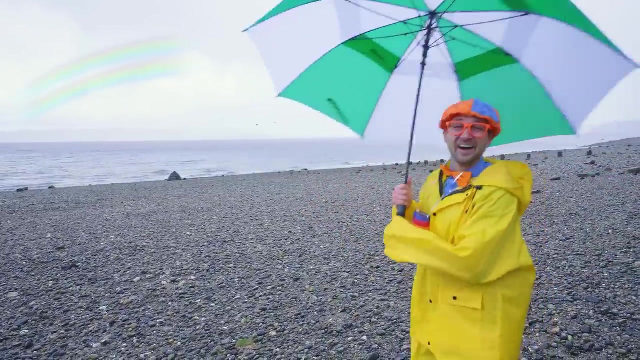 Yeah, a rainbow is an arch of colors made by light and water. Let's see if we can find one. Oh, Oh, Oh, Oh, Oh. a rainbow, oh, a double rainbow, oh, oh, oh, it's full on, oh, even a triple rainbow. 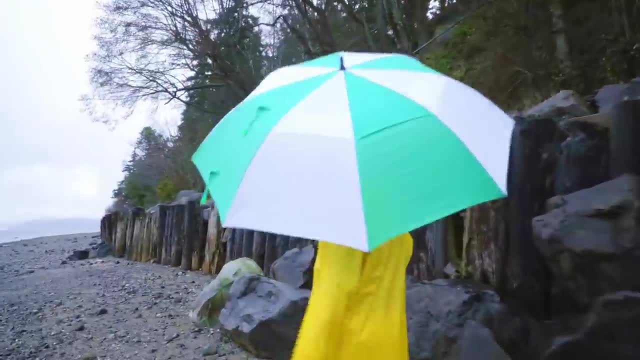 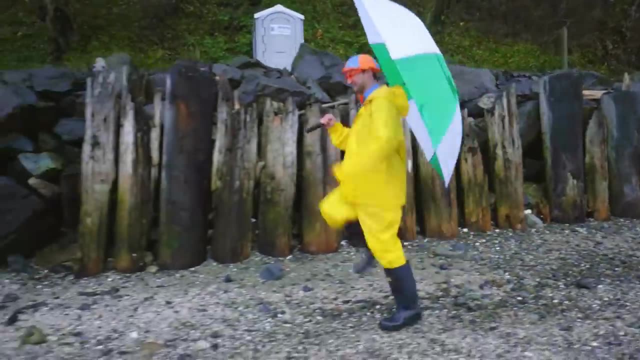 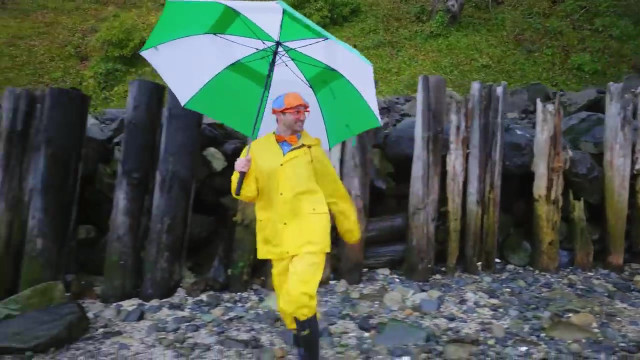 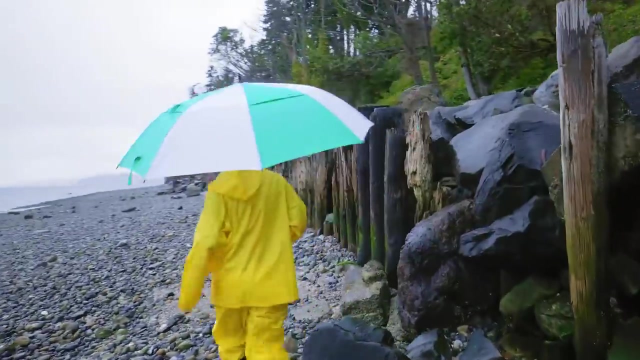 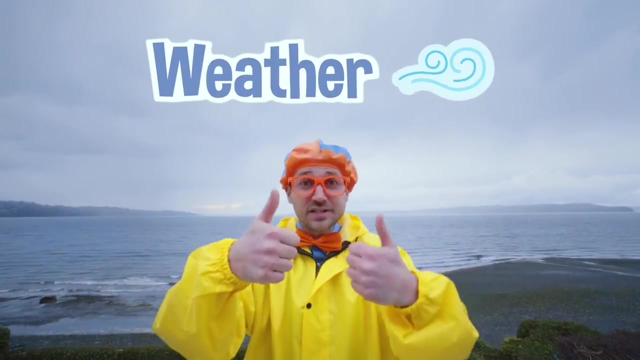 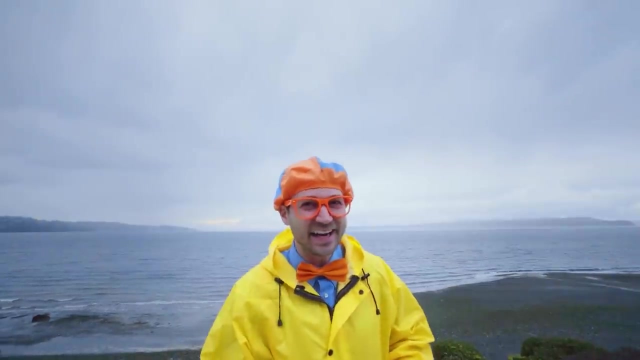 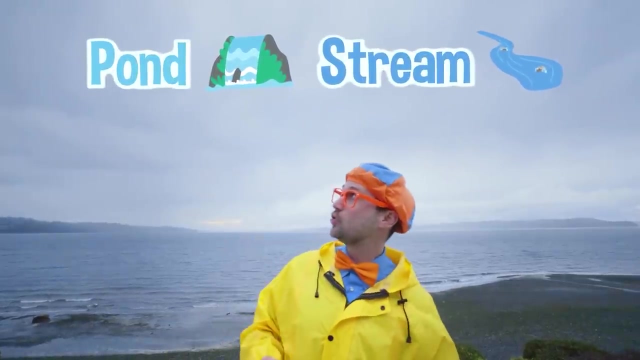 Oh a rainbow. Woohoohoohoo, It's a rainbow. Oh a rainbow. This weather has been awesome, Yeah, Hey, have you ever wondered where does rain come from? Well, let me tell ya. Okay, let's start with water in a pond or a stream or the ocean. 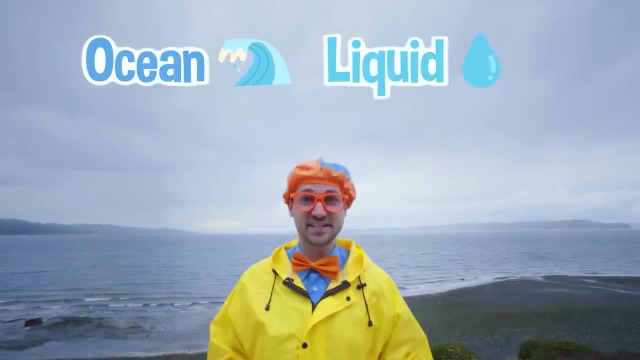 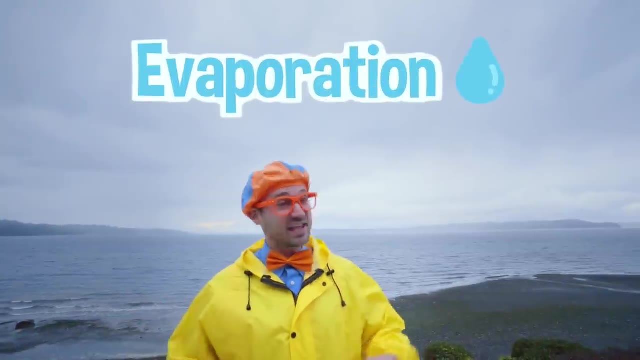 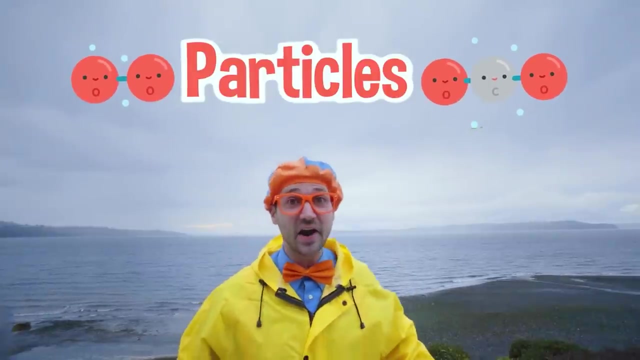 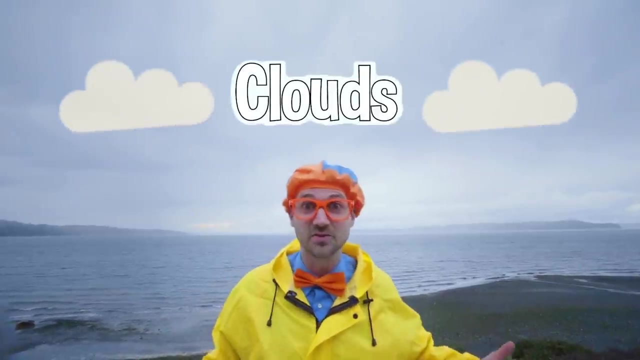 Yeah, water is a liquid at this time and place. And then water goes, what's called evaporation. Yeah, evaporation is when the water becomes these little tiny particles and goes up in the air. Yeah, it turns into a gas, goes up in the air and then turns into some clouds. 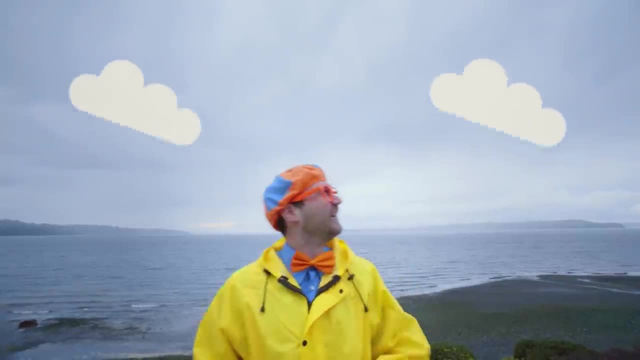 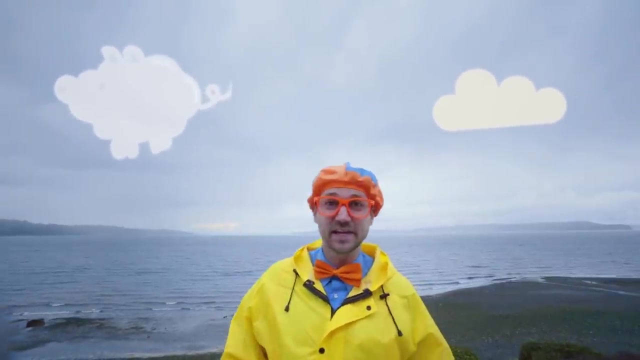 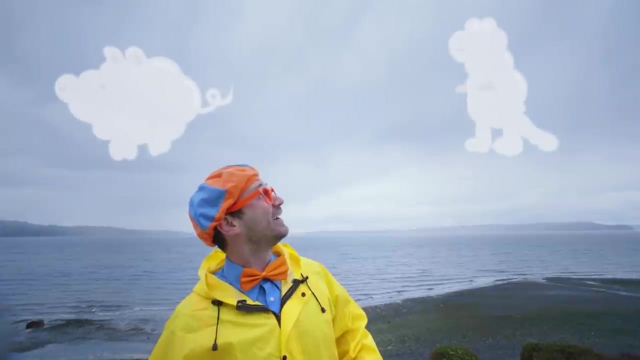 Whoa Yeah, Clouds are awesome. Whoa. look at that cloud. That cloud looks like a piggy. Oink, oink, oink, oink, oink oink. Look at that cloud. That cloud looks like a T-Rex. 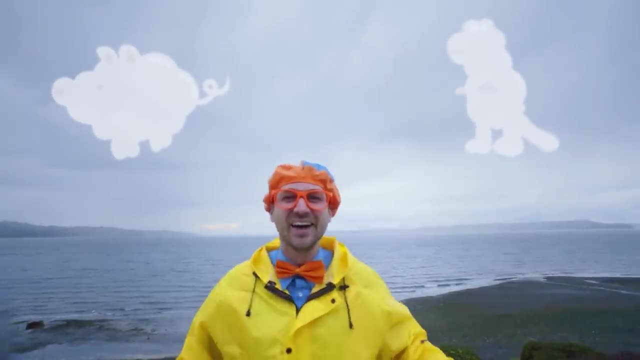 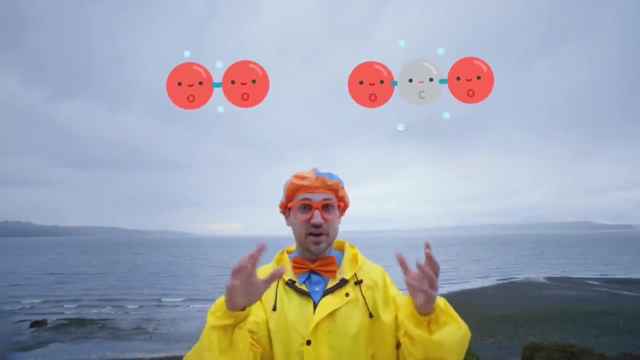 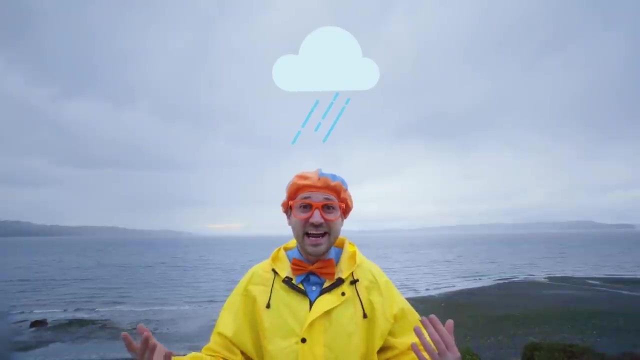 Wow, Wow. And then all this gas water starts to come closer and closer and closer, Yeah, and those clouds start to form into liquid water again, Yeah, and then rain starts to fall. Woohoo, Yeah, it's raining. 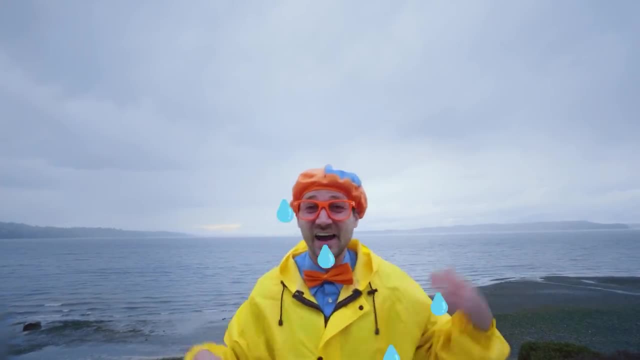 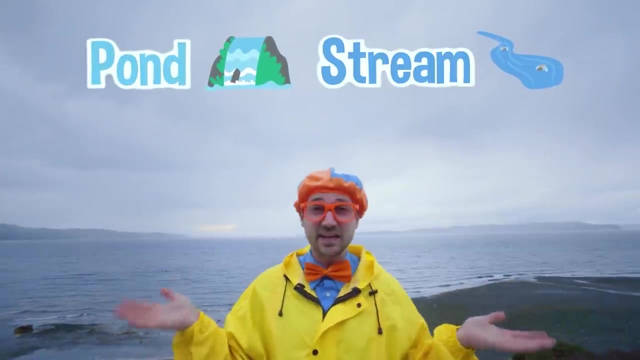 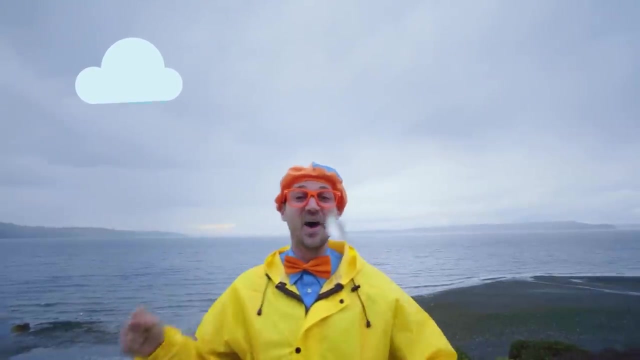 Whoa. And then they create puddles and streams and ponds and the water goes back into the ocean again. And then the cycle goes over and over and again and again. Wow, that water cycle is so great, Woohoo. 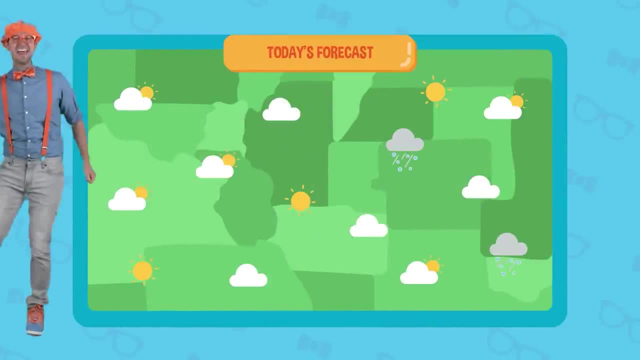 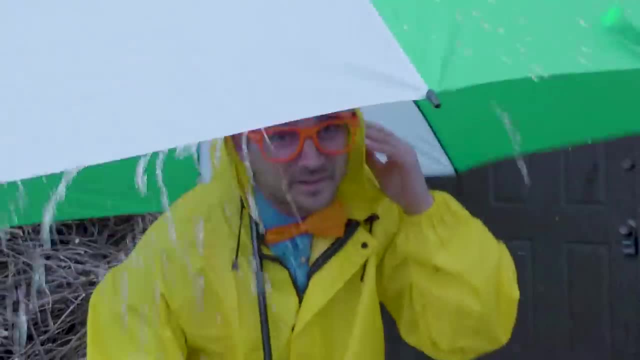 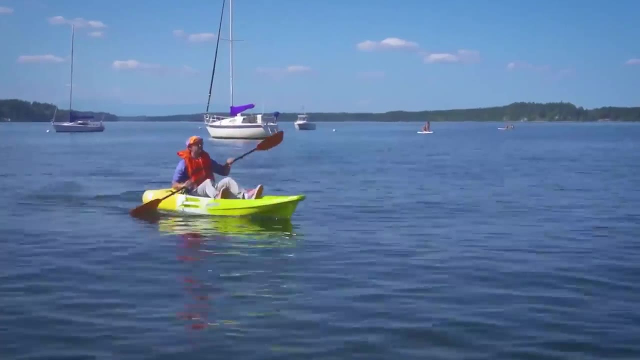 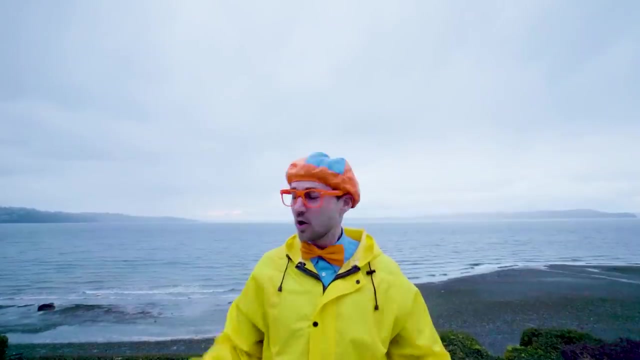 All the way in the afternoon. All the way in the afternoon. Don't forget your umbrella. The morning looks nice- Lots of sunshine, clouds of white and a bright blue sky- But the sky's turning grey. there's wind and some rain. 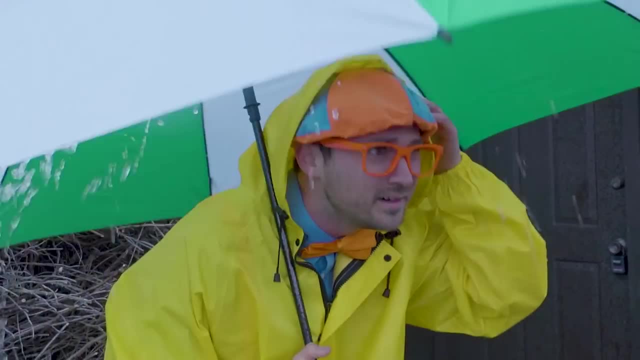 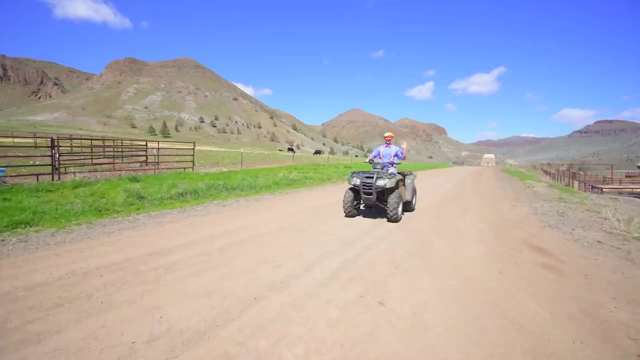 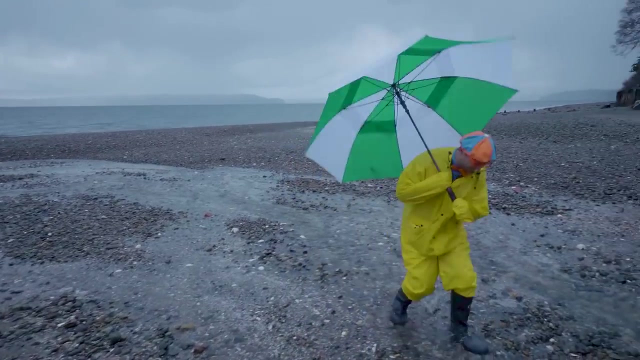 It looks like it's gonna be a stormy day. Weather weather- all kinds of weather- And some rain And some rain And some rain. Weather like sunny, breezy, cloudy, warm, pleasant days. Weather weather- all kinds of weather- like windy, rainy, stormy, hot, muggy days. 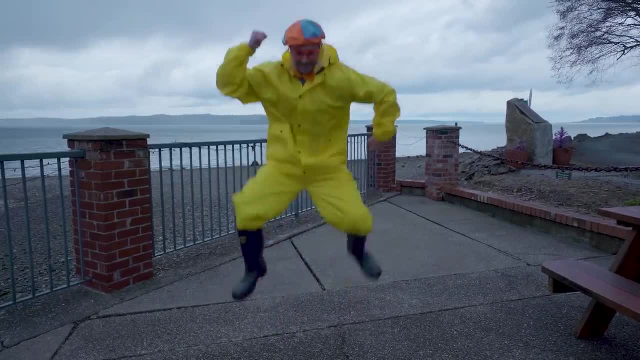 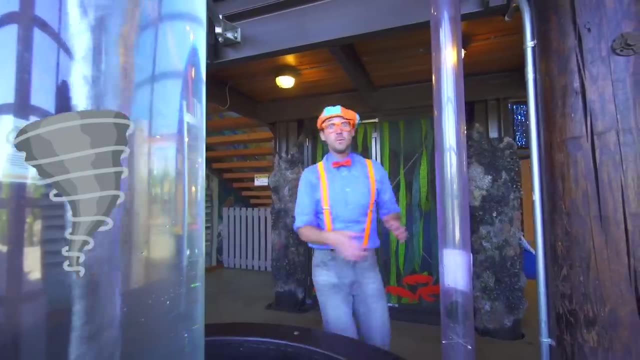 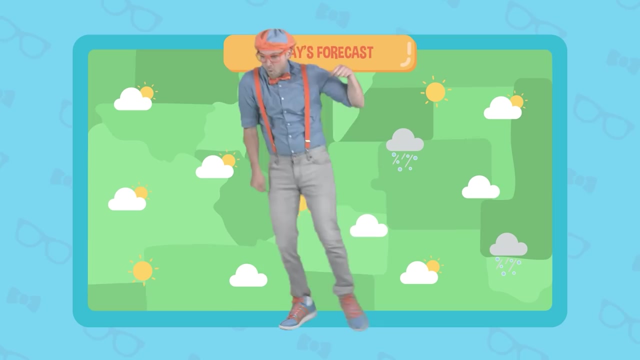 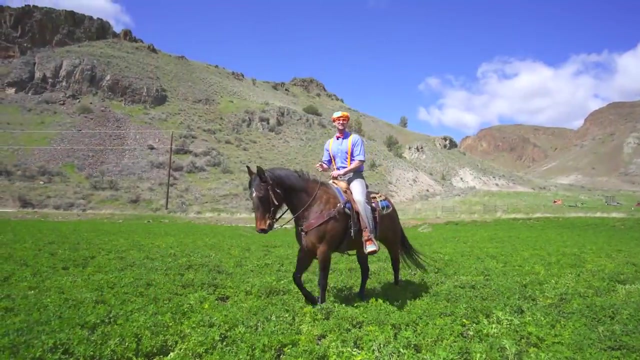 A lightning bolt, that thundering sound. there's a storm coming any moment now: Tornadoes, hurricanes and floods. sometimes weather can be dangerous Weather weather, all kinds of weather, like sunny, breezy, cloudy, warm, pleasant days. 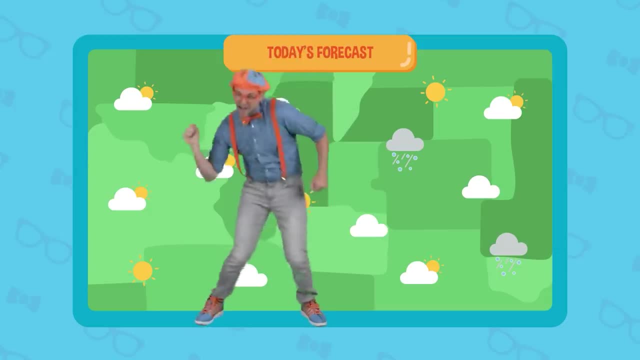 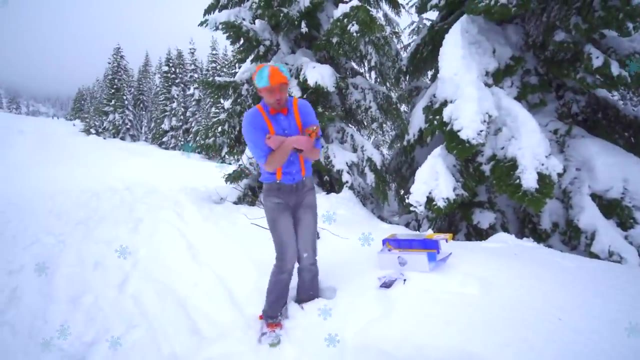 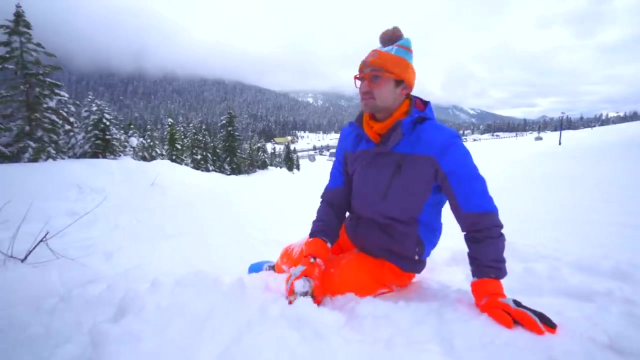 Weather weather. all kinds of weather like windy, rainy, stormy, hot, muggy days, And when it's really really cold, snowflakes will fall from the sky, Everything goes quiet and everything is covered in white. 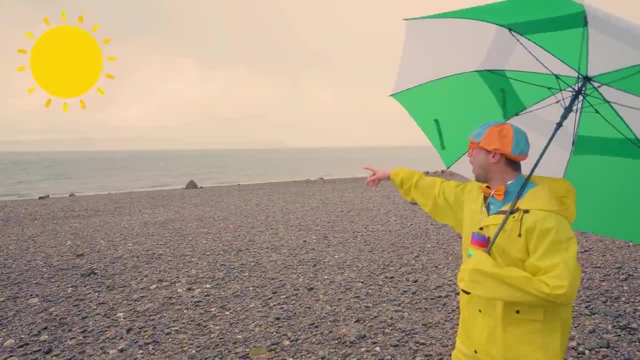 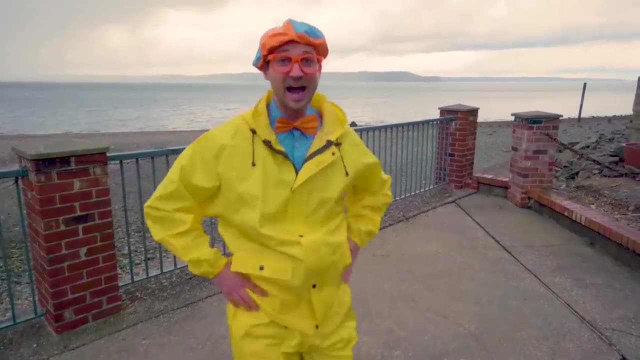 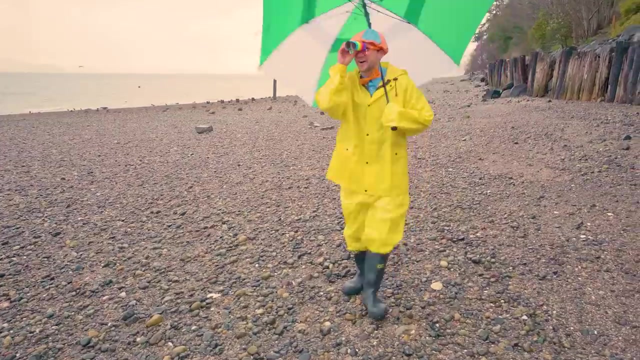 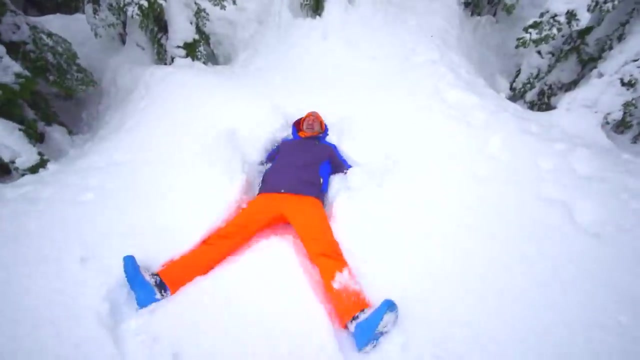 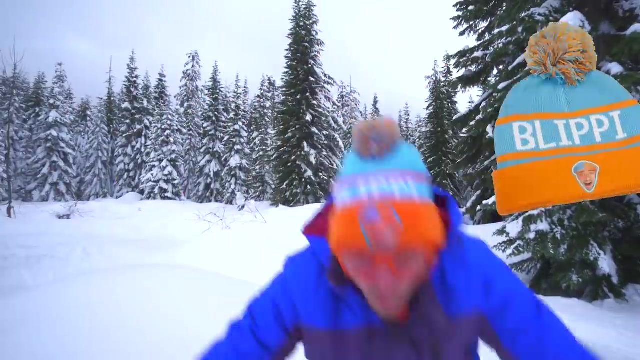 Hey, The rain has stopped and the sun's shining again. Weather weather- all kinds of weather like snowy, icy, blizzard, cold, frigid days. Weather weather- all kinds of weather like sunny, breezy, cloudy, hot, muggy days. 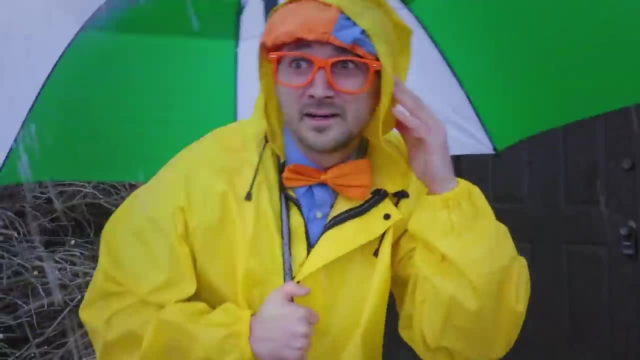 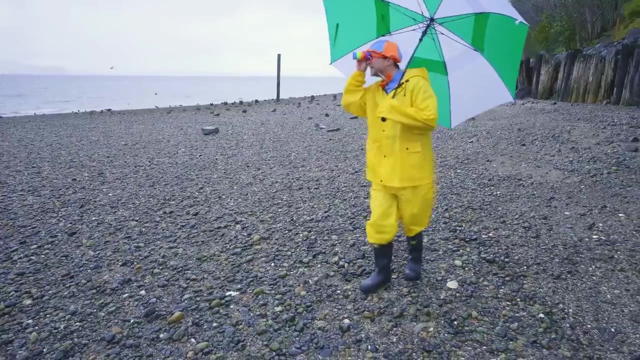 Well, this is the end of this video, But if you want to watch more of my videos, all you have to do is search for my name. Will you spell my name with me? Ready B-L-I-P-P-I, Flippy. 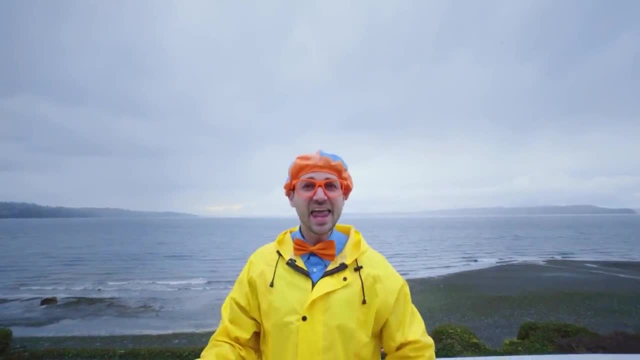 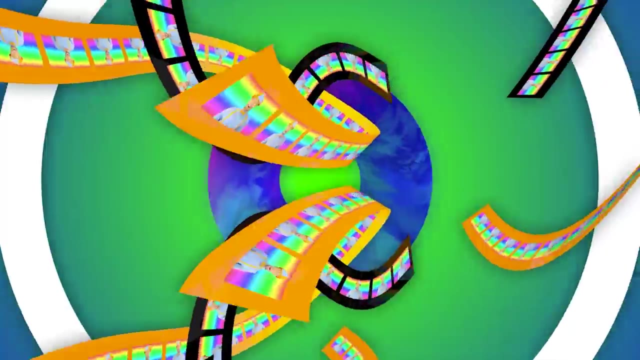 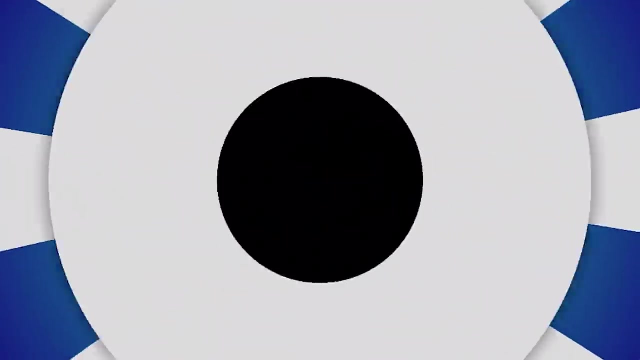 Good job, All right, See you later. Bye, Flippy. Come on everyone, Let's make learning fun. Blippy, Blippy. So much to learn about. It'll make you want to shout, Flippy.